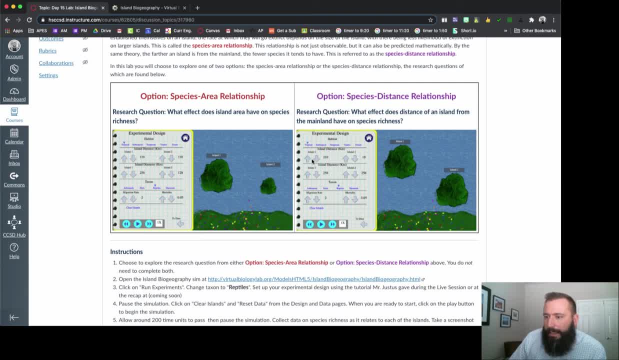 design. Notice that the island distance from the mainland is the only thing along the map that's being studied In this particular equation. here we've got six islands in thisард cancer and to the left three, means that is different between all of the other, between these two islands, So all of those other. 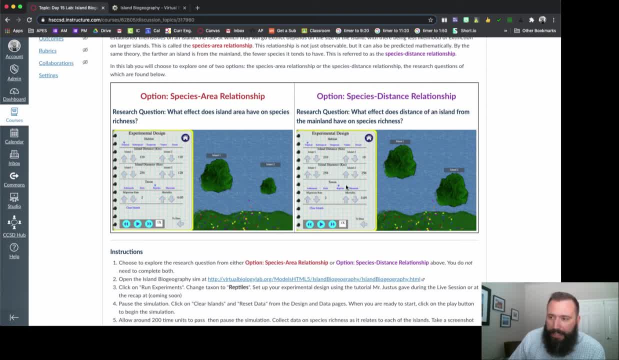 factors like island area, the taxon, the migration rate, mortality rate and even the habitat are all the same between the two islands, except for that one factor that we're changing, that we're manipulating that independent variable right, Whether that's island area or distance of the 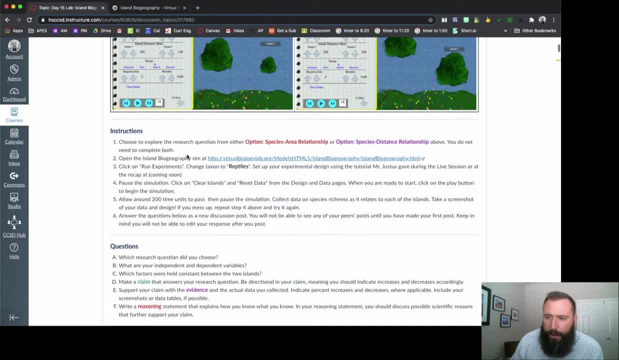 island from the mainland. So, look, I've read out some instructions for you to further help you out. So you're going to choose the research question, the one on the left or the one on the right. You do not need to complete both. Open up that sim in a moment And in a second I'm going. 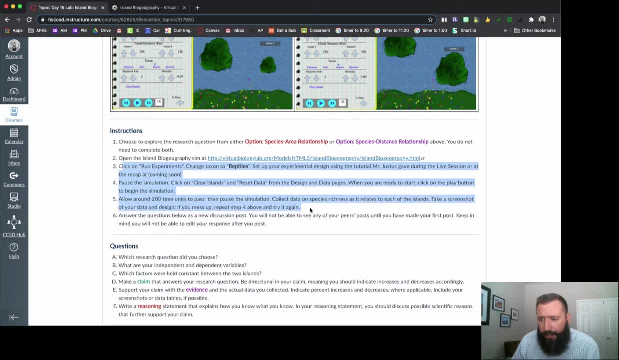 to walk you through those instructions here. So if you get lost along the way, just know that the instructions that I'm going to explain using the sim are also here on available for you on our Canvas page, all right, So we're all trying to. just real quick, take a look, We're trying to. 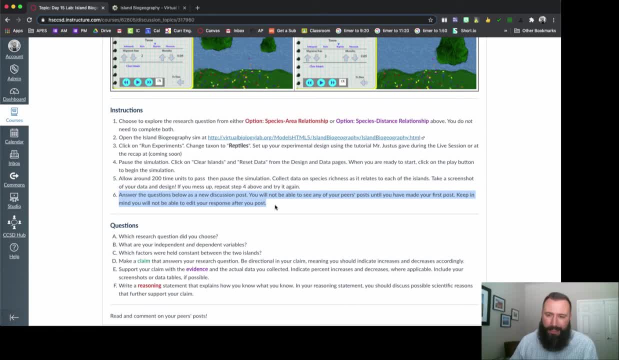 create a discussion post With this lab, all right, So you're going to answer the questions below as a new discussion post. You're not going to be able to see your peers post until you've made your first one, and then you won't be able to edit your response after you post. So make sure that we are collecting our data and 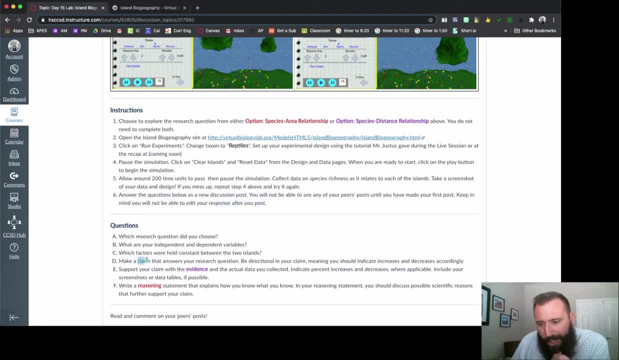 really careful when we're answering those questions here, right? Notice? I'll just point this out. right, We're going to be answering a claim supported by our evidence with some sound reasoning that helps support that claim. all right, Yeah, there's going to, you know, identify the independent and. 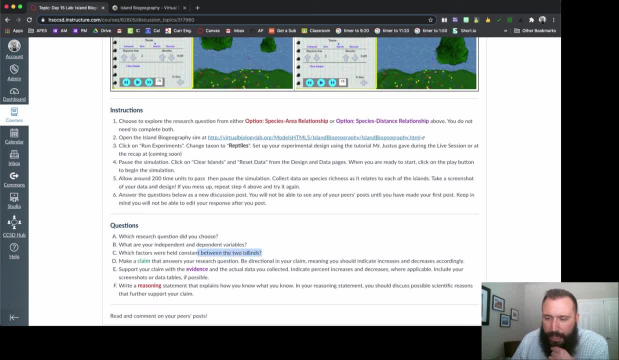 dependent variables. You'll tell me about the research question you chose and also those factors that you hold constant between the two different islands. But let's go over to the simulation, because I think that will clear up some of the confusion you might have about this. So this is what it looks like here When you first actually open it up. let me 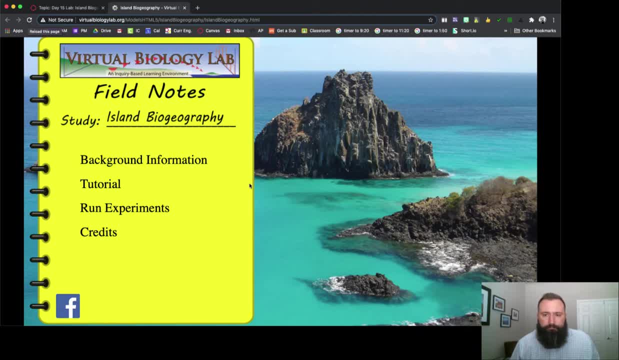 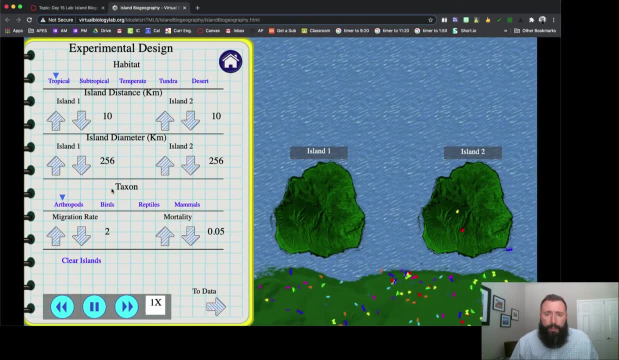 just refresh it So to show you what it'll look like when you open. The link that we care about here is run experiments, so we'll do that Right away. notice that the very first thing I tell you to do is change the taxon. 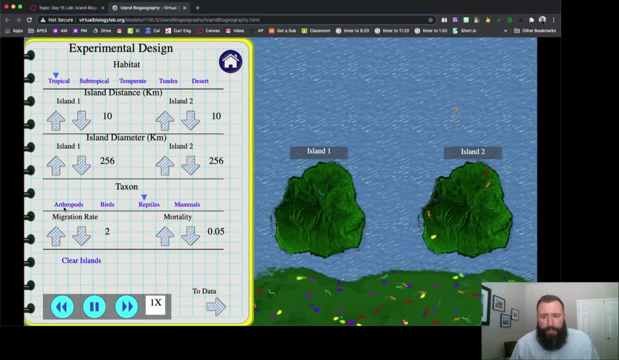 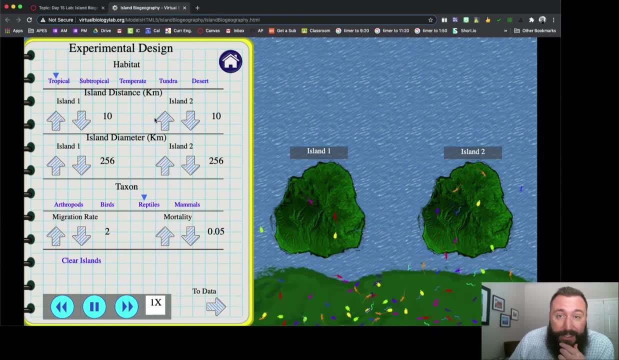 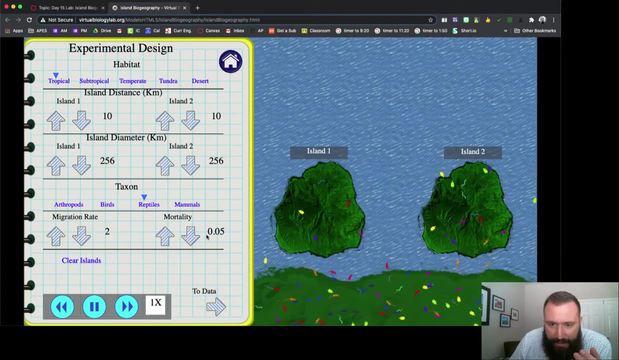 on to reptiles. all right, Just like that. all right, We'll get some better results because of that. Now, if I'm interested in the species distance relationship, that means I'm first. I'm not going to change the diameter, the taxon, the migration rate, mortality or habitat. the only thing I'll do is change the distance. 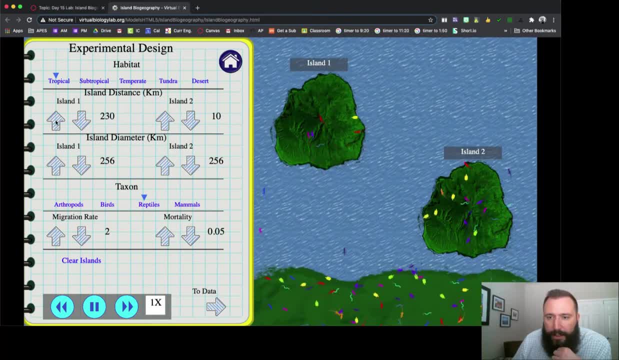 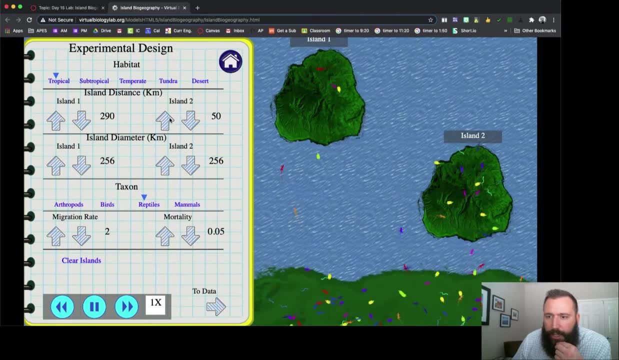 So what I'll do is just push one of these islands, island one, out into the ocean a little bit more. and what if I just push 2 out just a little bit too? I noticed that the simulation is running, so push, pause, right. 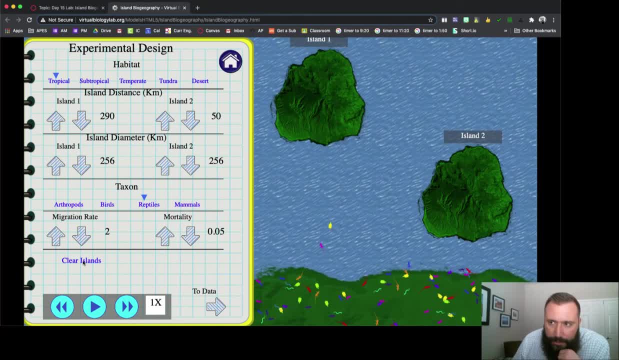 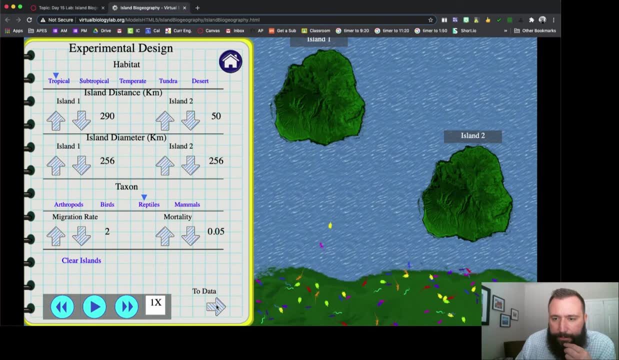 In fact. take a look, See this: clear islands. Every time I do this, if I want to make a change, I just push pause in that simulation and then click out clear islands. Take a look, There's another way that we can reset it too, So I'm going to go over to the data section. Notice that I can. 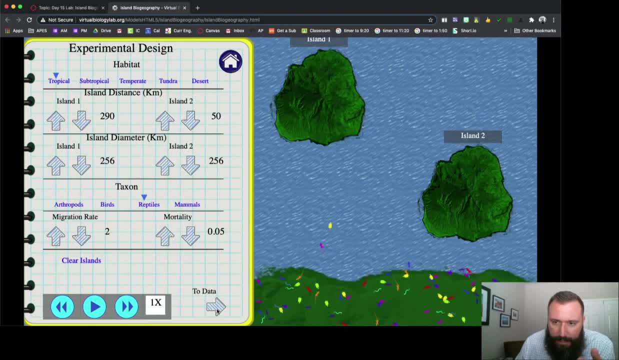 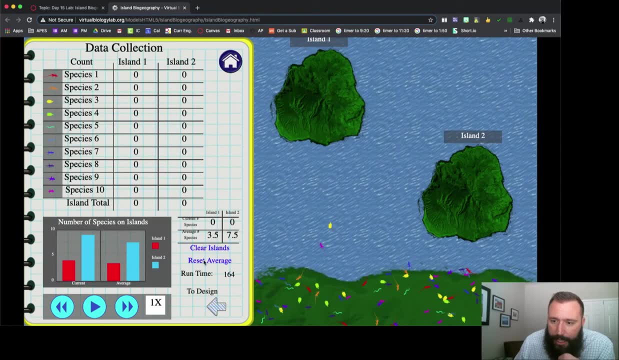 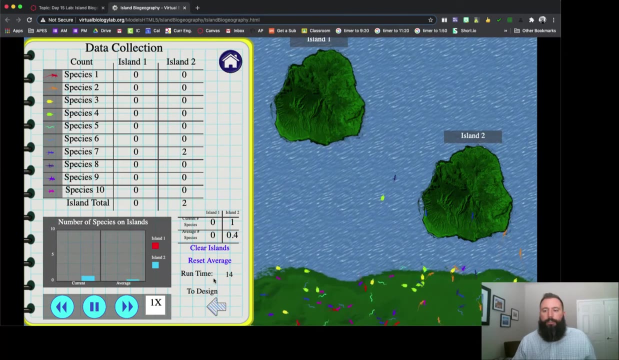 toggle between my design and my data with the button right here in the lower right of this area, right, So take a look. Hey, I want to reset the average too, so click on that. Notice it doesn't just go away. I need to push start in order for it to kind of reset. So it's moving. 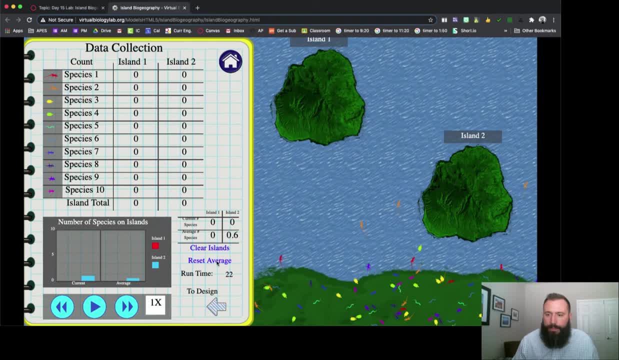 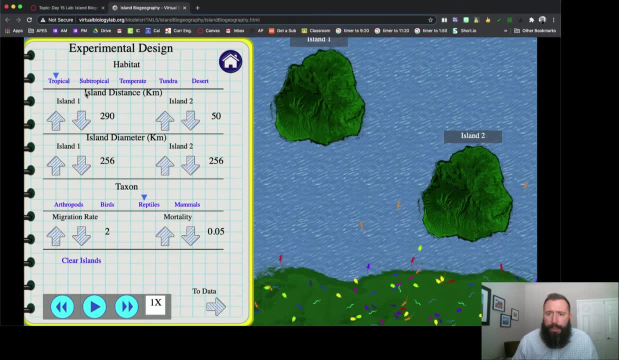 I'm going to push pause. I'll click clear islands and I'll click reset average. all right, Okay, so let's go back over here. It looks like I've got I'm all set up right. I'm interested in. 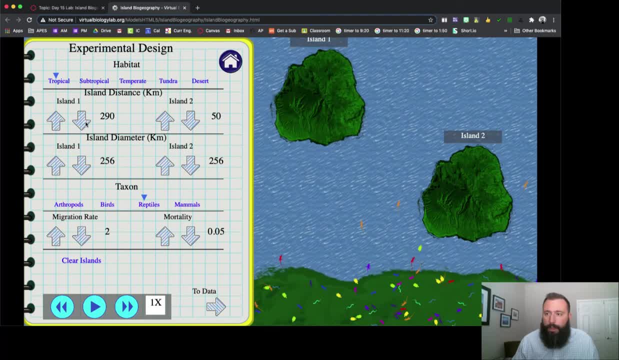 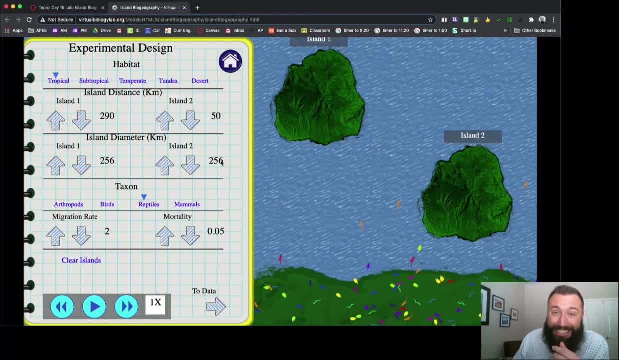 species distance. One of the islands is further out than the other, but all of the other parameters are being controlled. That way we can really determine whether or not distance is what's changing that species richness right, Our dependent variable. So when I'm ready to go, I'm going to push. make sure I 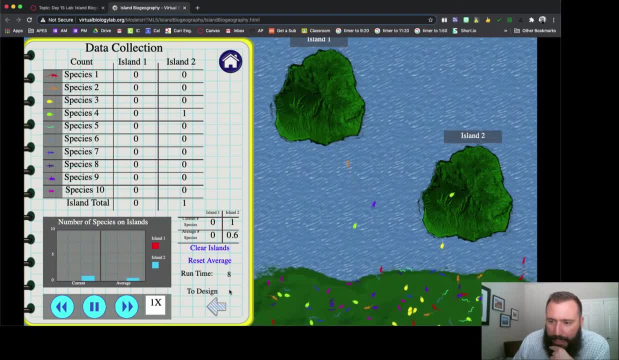 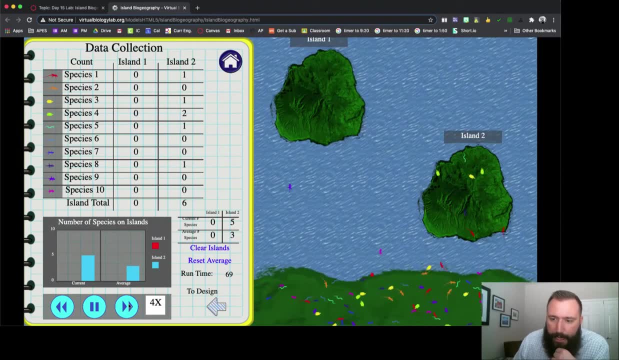 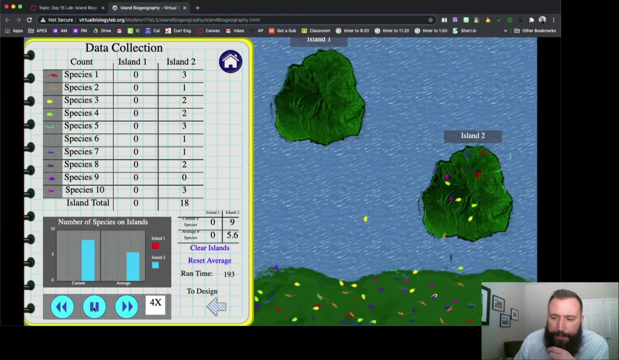 clear islands, reset average and then push, play And then time units will start ticking away And what we'll do- we can actually speed up this process a little bit. What I'd like to do is to go to 200 time units, Allow that 200 time unit seconds to pass, whatever this time is- and push. 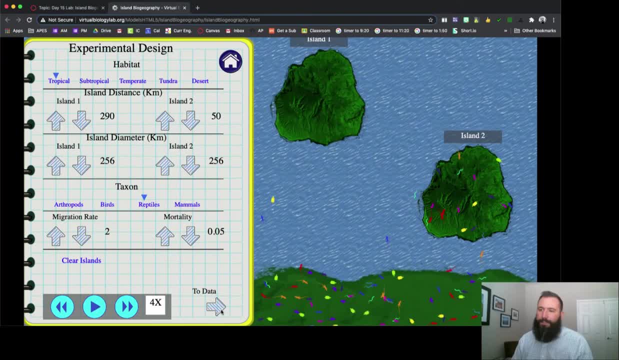 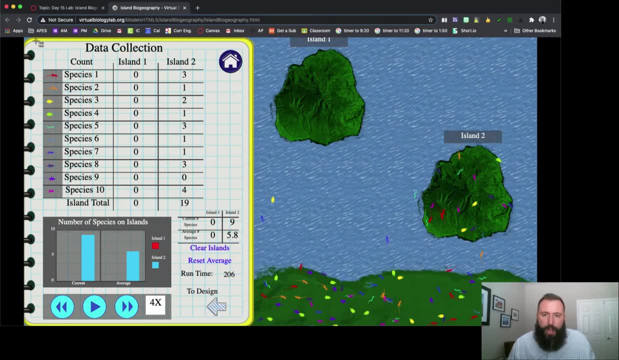 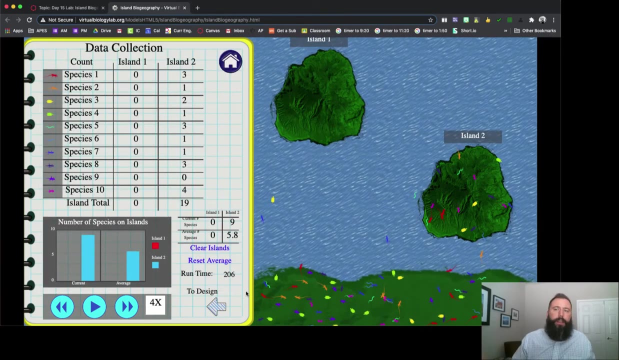 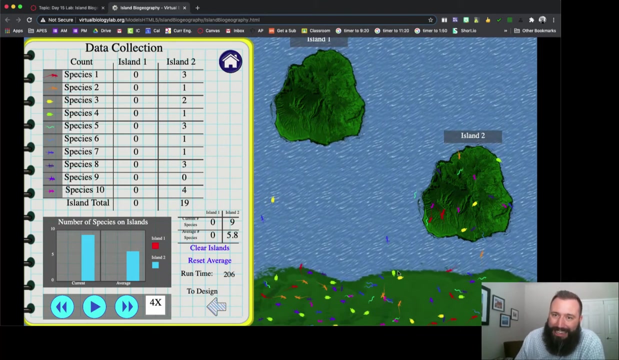 pause If you're not exactly on 200, it's fine. Right there, we can start to make some claims, okay, So what I'd like you guys to do, actually, is make a screenshot of the data table, And I just I'm using my screenshot tool on my Mac computer. It's going to be different for yours- Google screenshot Chromebook or screenshot Windows. if you don't know how to do that, I'll be able to take this data and incorporate it into my post. all right, If I wanted to do it again, or maybe even find averages between trials, I'll click. 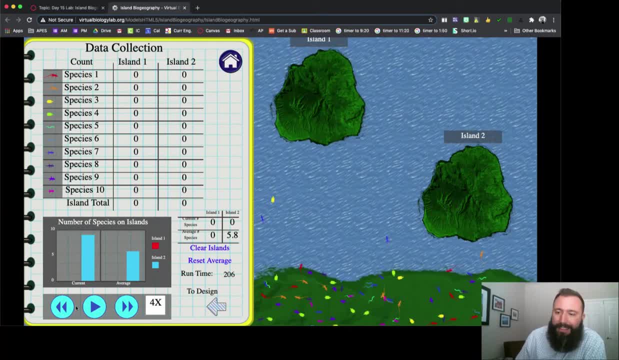 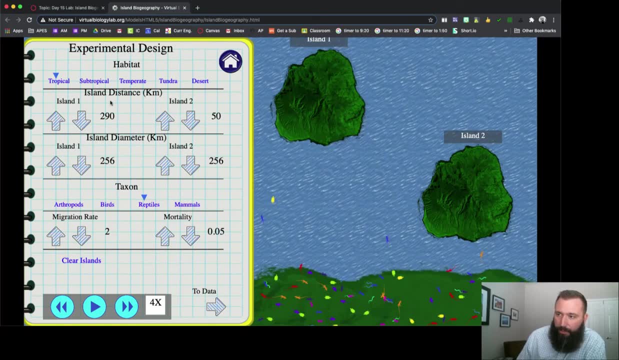 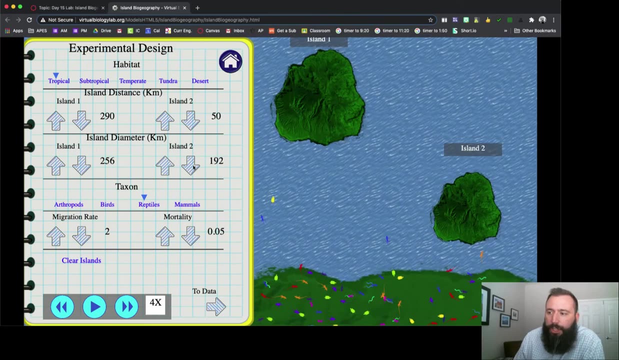 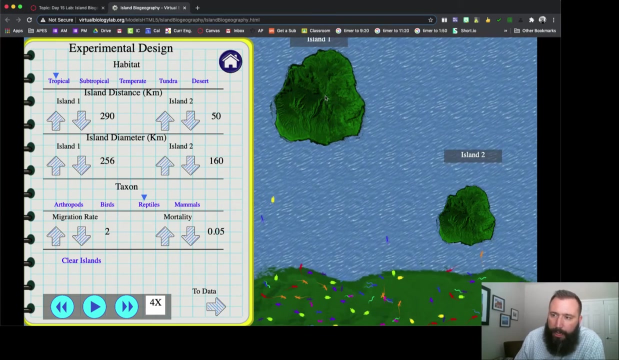 pause, I'll click clear islands, reset average and I can do it again Now. yeah, this is if I was interested in the species distance relationship. If I was interested in the species area relationship, my experimental design will look a little bit different. What I'd want to do is I'd want to change one of the islands and make the area a little bit smaller. This other one island one will leave a little bit bigger, But remember, we're testing out area, So I want to keep all of those other variables then the same. 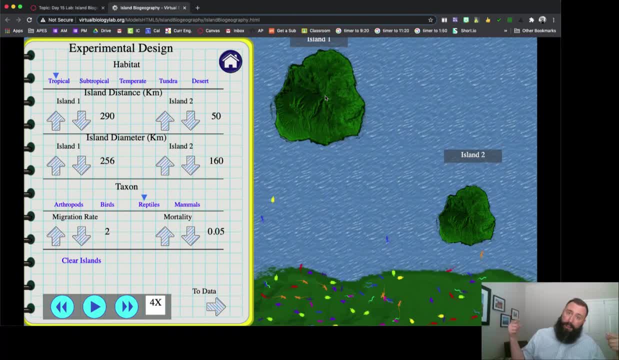 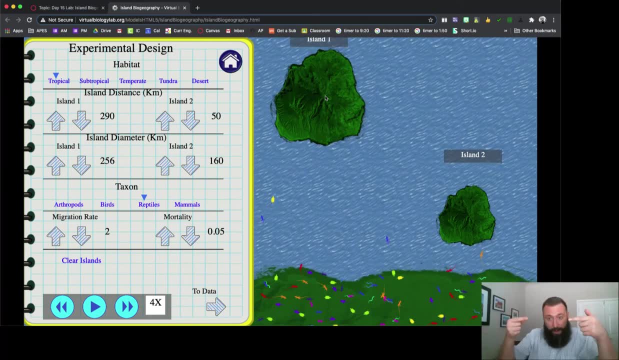 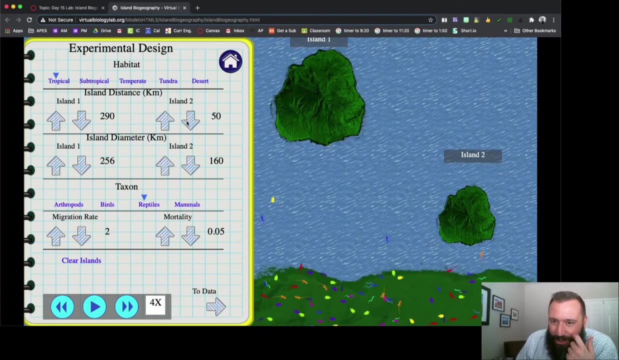 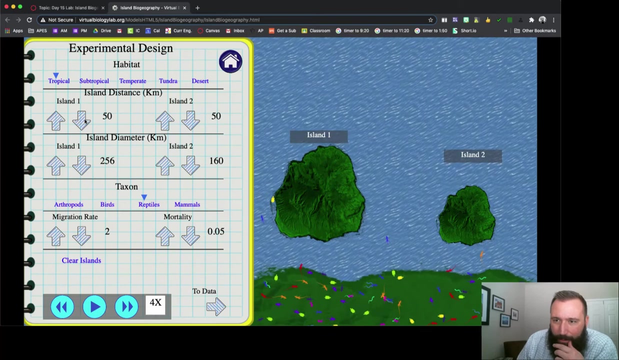 Right. Last time I had area constant when I was testing out distance. Now I'm going to keep area different and keep area distance constant, if that makes sense. So I've got different diameters here of different areas, but I want to make sure that the distance from the mainland is the same for each of these islands. So let's get them both up to be about 50 or so, All right? Hey, area is different, Distance is the same. I want to make sure that the distance from the mainland is the same for each of these islands. 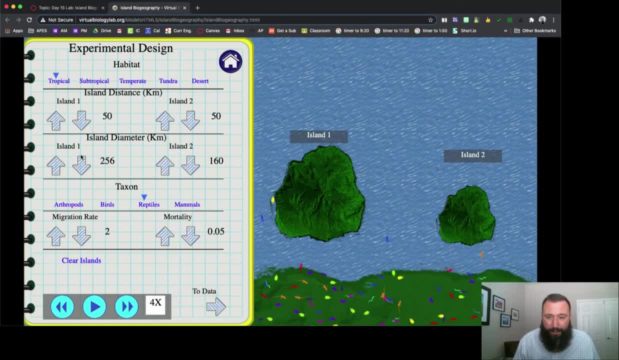 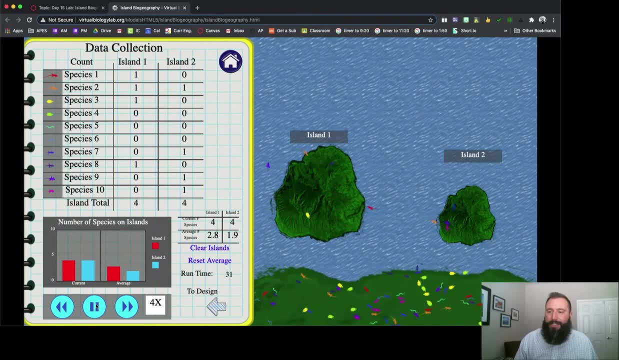 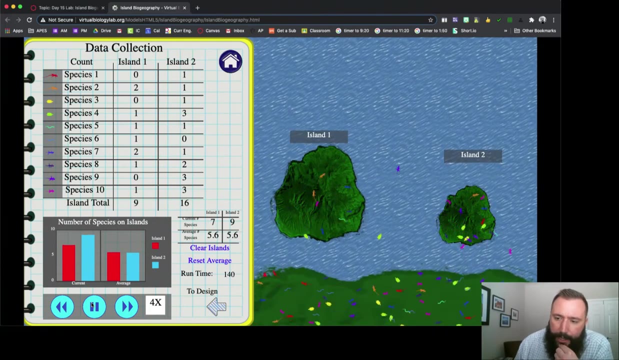 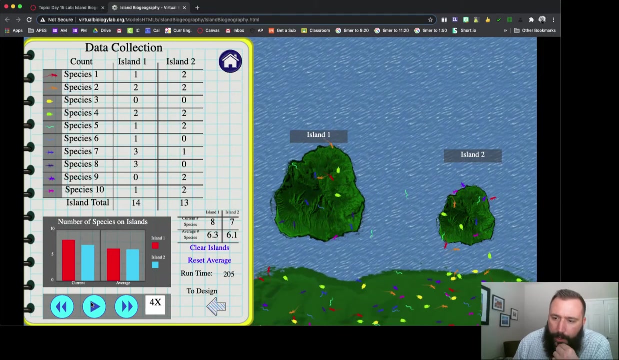 Make sure that my taxon is reptiles. Migration rate, mortality is the same. Habitat didn't change. Let's clear islands. Click reset average and we'll let the process go again. We'll allow 200 time units to pass. After 200 time units pass, I will push pause. All right, And there we go. Okay, So at this point we will be able to collect some data.